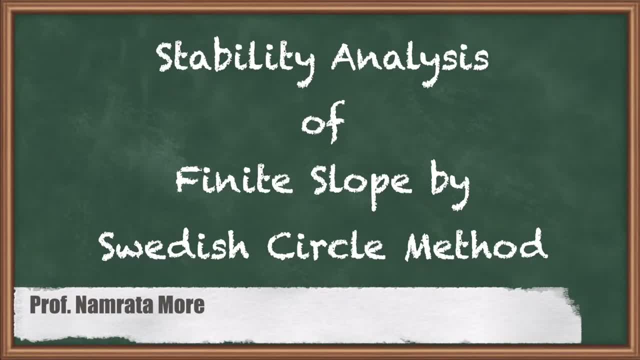 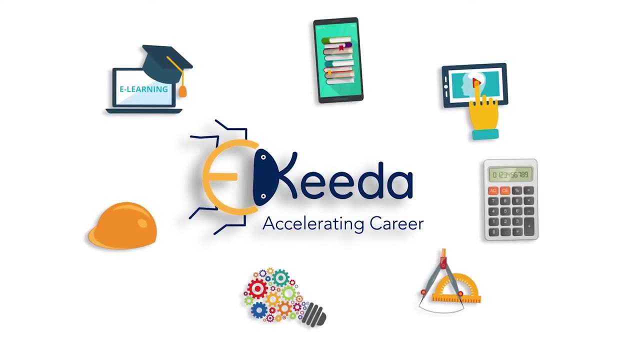 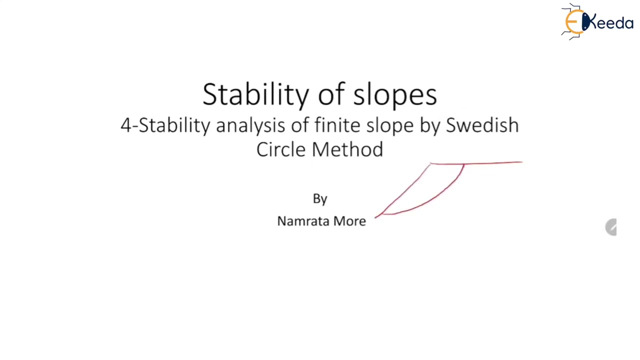 Hello everyone, in this video we are going to discuss Stability Analysis of Finite Slopes by Swedish Circle Method from the chapter Stability of Slope. So, in short, in this video we are going to assume a trial failure surface and for this surface we are going to determine the factors which causes overturning. 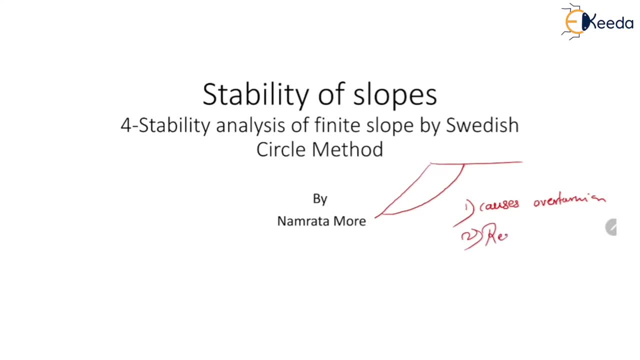 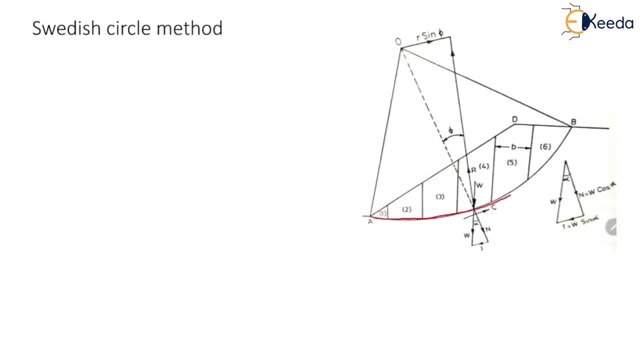 We are going to discuss the factor which raises the slope, Resist, overturning, and then, by using this knowledge, we are going to determine the factor of safety for that slope. So let us consider AB as a trial circular failure surface. So the radius of this circular failure surface is R and center is O. 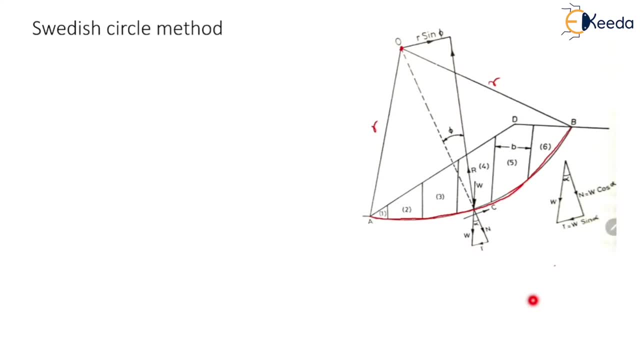 The wedge which is above this failure surface is D. This wedge is divided into vertical slices. So this wedge is divided into vertical slices by drawing vertical line. So in case of homogeneous soil these wedges are of equal width. But if the soil is non-homogeneous, then in that case suppose this slip surface is passing through more than one type of material. 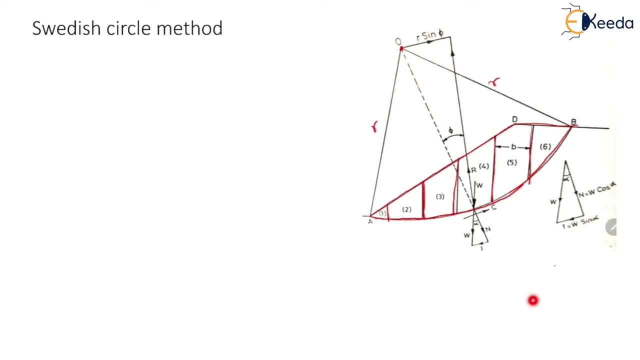 Then this vertical line will be present At the junction of that two materials, Means that condition will depend- will govern the width of this slice. These slices are in equilibrium under following forces: The first force is weight of each slice, denoted as W. 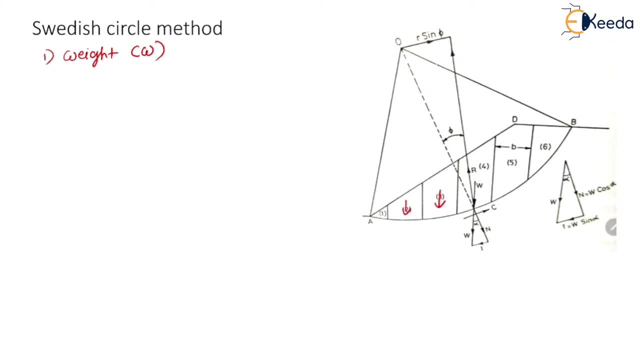 It acts in vertically downward direction Through the center of gravity. So these are the. this is the first force acting on the slices. Second force is cohesive force, denoted as C. This force acts along the curved surface in the direction of probable movement of the wedge. 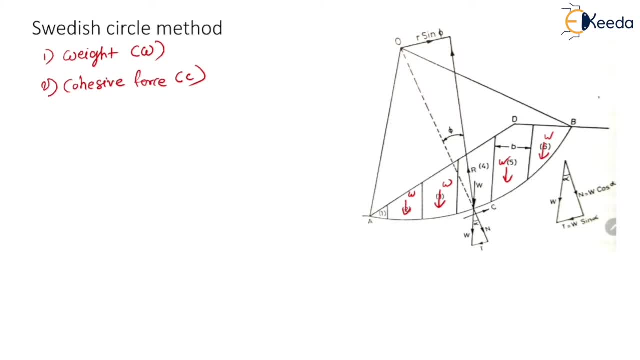 So suppose, because of slippage, the wedge is moving In downward direction, Then cohesive force will act in upward direction Because it will try to resist the movement of the wedge. So for each slice cohesive force will be acting in upward direction Along the curved surface. 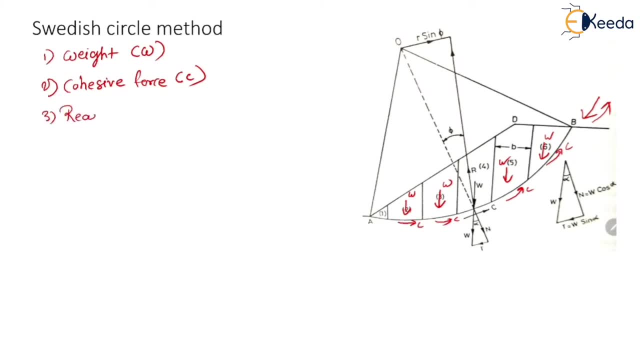 The third force is reaction R. At the base It is inclined at an angle phi to the normal. So suppose, if we draw a normal for each slice, Then this reaction R will be inclined at angle phi to the normal. Means angle between reaction and normal to the slip surface will be phi dash. 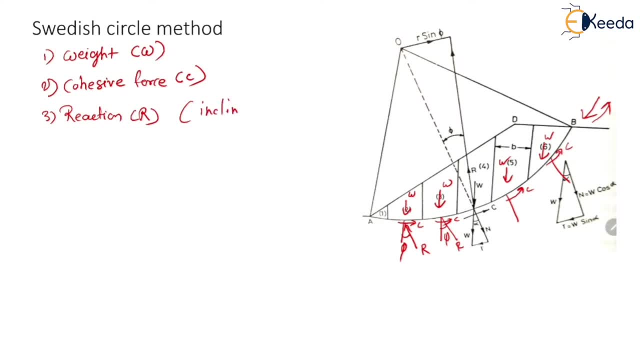 So reaction is inclined At an angle phi to the normal And the fourth force will be reaction of two vertical sides of slice Due to Adjacent Slices. So suppose this is an intermediate slice, Then because of the adjacent slices, 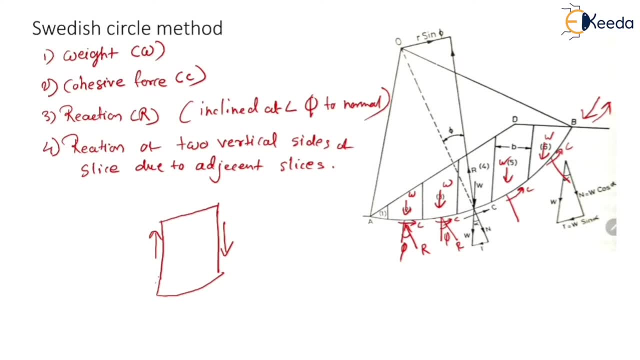 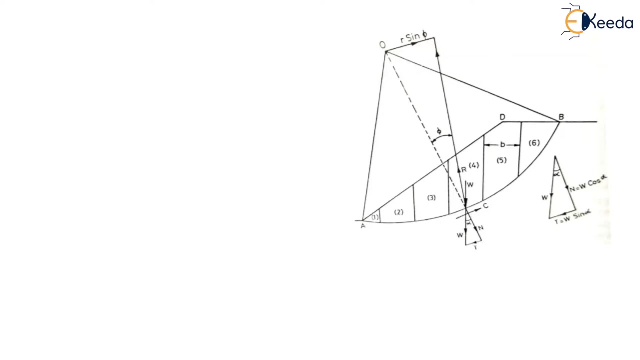 There will be reaction on both the sides of the slices, And these reactions will be in opposite direction and equal in magnitude. That's why they will Cancel each other And hence they are not considered to affect the stability of the slice. For convenience, let us consider the equilibrium of the single slice. 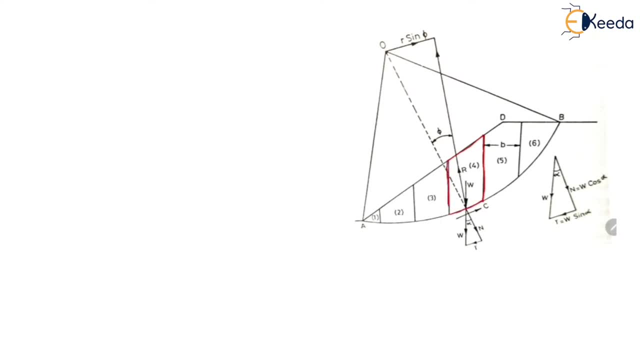 Now let us consider this slice number four. So the force Acting on this slice is W, Which is acting in downward direction. So this force can be Resolved into two components. First component is along the Normal to the Slip surface and second is: 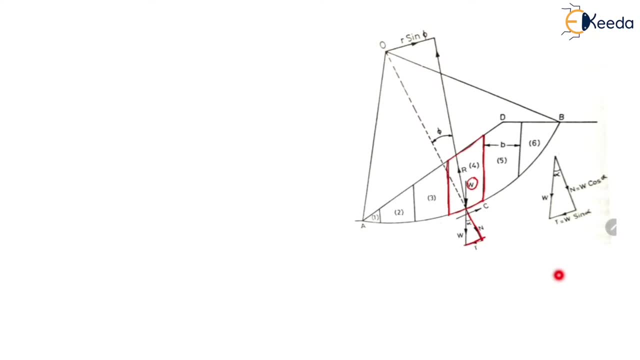 Tangential to The slip surface. So Here we can see a larger view of this forced angle. So W acting in vertically downward direction. Here N indicates the direction of normal to the slip surface. So angle between W and N is: 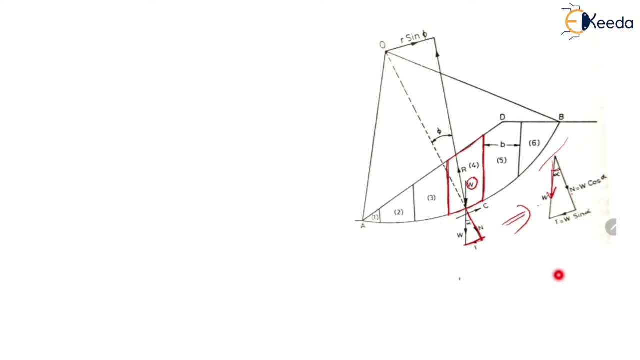 Alpha. So from this figure we can see that Normal component of W is equal to W cos alpha And tangential component of W is W sin alpha. The another force acting on this slice is cohesive force C. It is acting in upward direction. 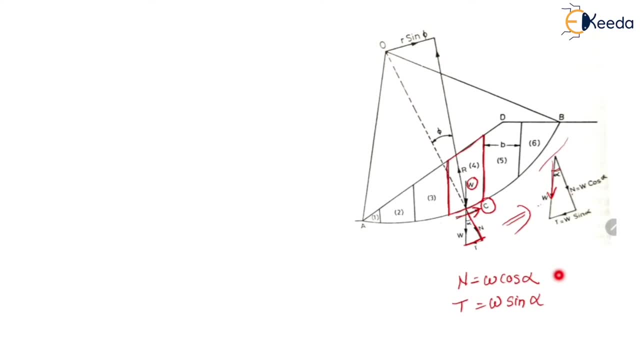 As this wedge is trying to slide In downward direction. And the third force Which is acting on this slice is Reaction R. Now, as we have discussed That, this reaction R Makes an angle phi with the normal. So here, 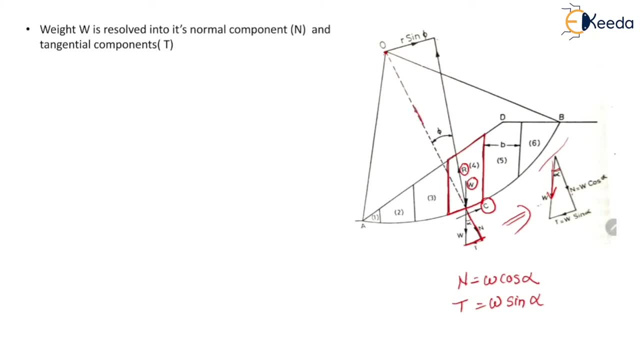 This Hash Dashed line Indicates the direction of Normal. Obviously it will pass through the Center, And here this line indicates The direction of reaction R. Now we will draw A line from point O, Such that 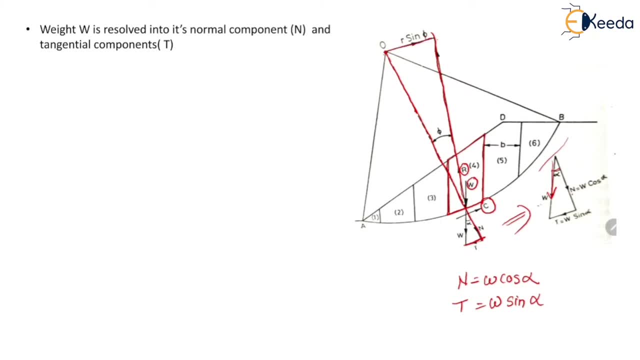 This line will be perpendicular to reaction R. So This line Which is passing through O, is perpendicular to the reaction R, So this distance will be equal to R sin phi. In short, If we draw A circle with center, 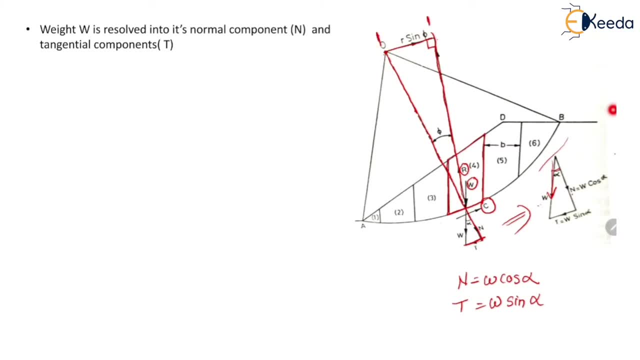 O And radius R sin phi, Then This reaction R Will be equal to R sin phi. In short, If we draw A circle with center O, Then Reaction R Will be tangential To this circle. 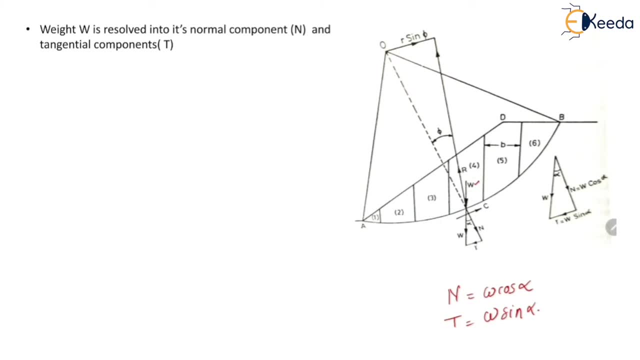 Now We have forces Acting on this page are W. W is resolved into two components: Normal component And tangential component. The remaining forces are Cohesive force C And reaction R. So If you want to take, 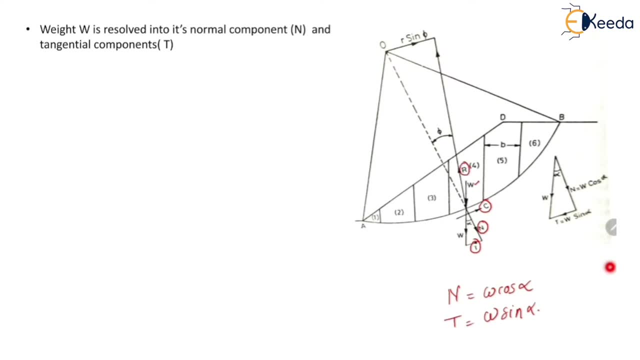 The movement of this Forces About this Center, Of this Failure. surface O, Then Reaction R, Then Normal Component Of N Won't cause any movement Because it is Passing through the Center. 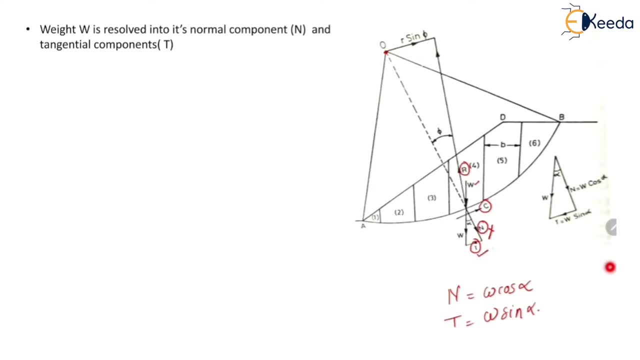 And Tangential Component Of Weight Will try to Cause Overturning And Cohesive Force Will try to Resist The Overturning. Similarly, This Reaction R Will also. 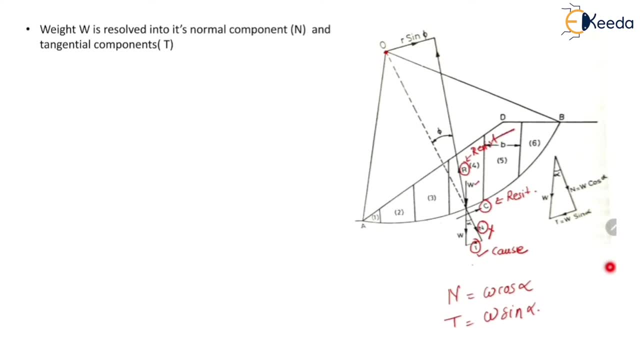 Try to Resist The Overturning. So Here T Is The Factor Which Try to Cause The Overturning And C And R Try to Resist The 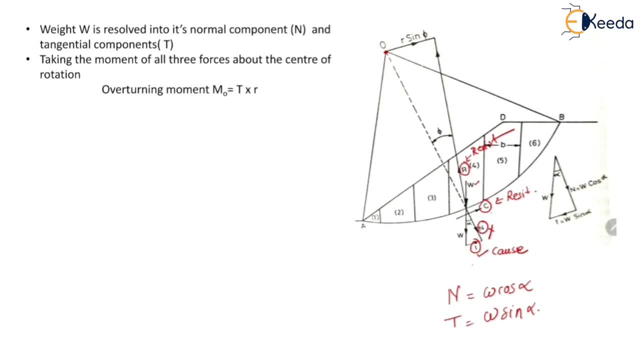 Overturning, So Taking The Movement Of All These Are From The O. So This Is The Overturning Movement And The Resisting Movement M. 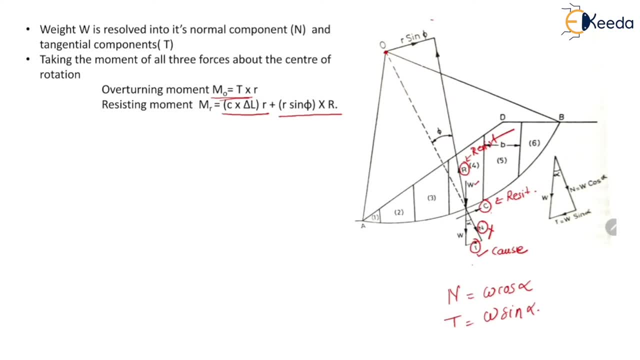 R Is Equal To Movement Due To Cohesive Force Plus Movement Due To Reaction R, Where R Is The Radius Of The Slip Surface Plus. 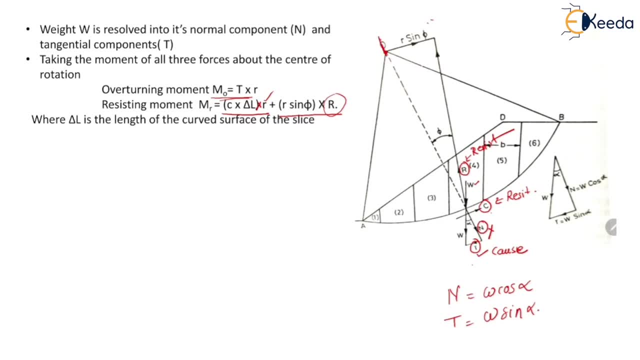 This Movement Due To Reaction R Is Equal To Reaction R Into This Radial Distance: Distance Between Reaction To R Now Resolving Force R Into. 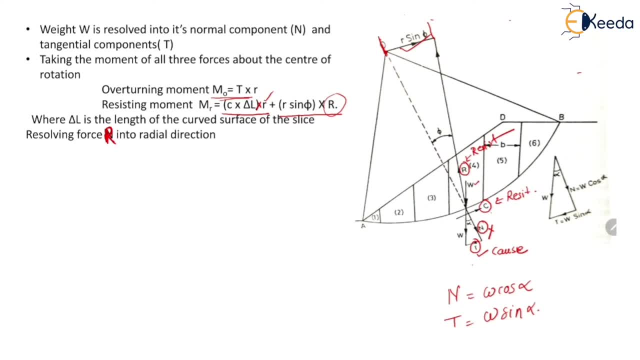 Radial Direction. So Here Normal N Is Also Acting In Radial Direction. So If We Resolve The Reaction R In Radial Direction, Which Right? 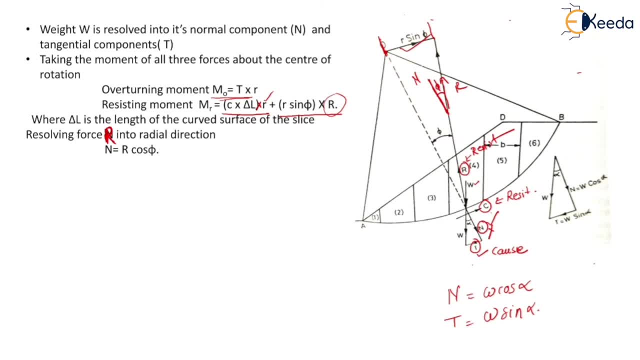 N Is Equal To R Cause 5.. That's Why R Is Equal To N Upon Cause 5.. Hence R Sign 5. Will Be Equal. 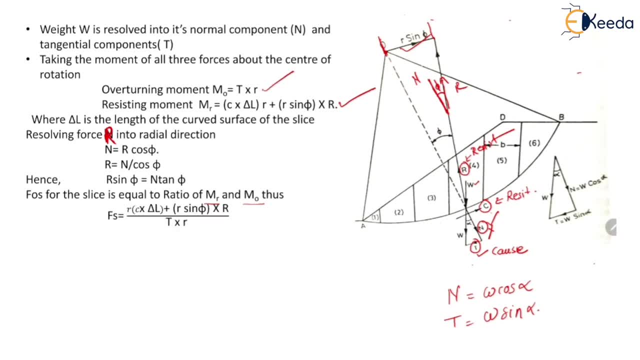 To N 10.. 5. Factor Of Safety Will Be Equal To Fs, Equal To R, Into C, Into Delta, L Plus R Sign 5.. 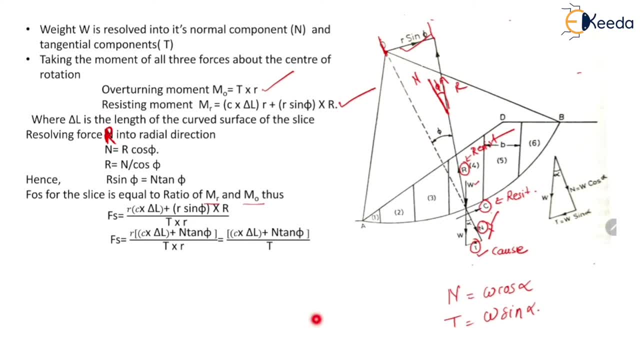 Into Capital, R Divided By T Into R, So R And R Got Canceled, So Factor Of Safety Is Equal To C Into Delta L. 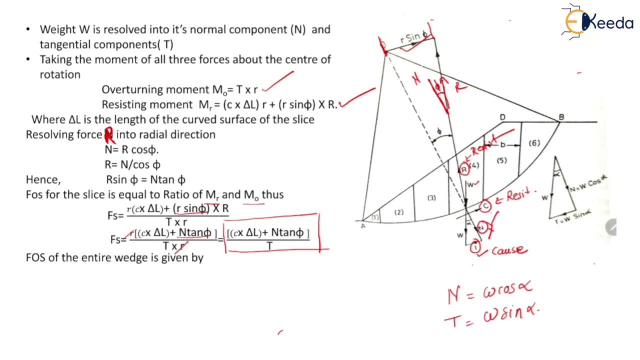 Plus N 10.. 5. Divided By T. So This Is The Equation For Tan Phi Into N Divided By Summation Of T We. 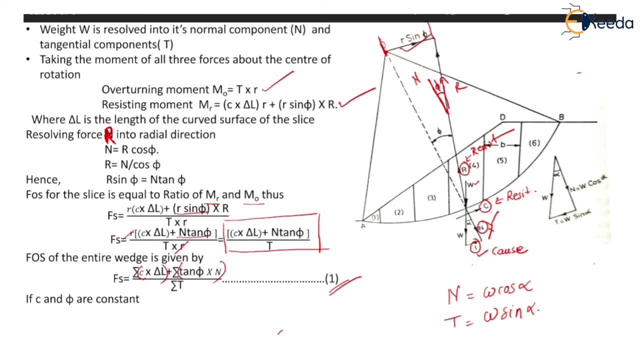 Will Name This Equation As Equation Number 1.. Given Slope, The Value Of C And Phi Are Constant. That's Here Tan Phi Is Constant. 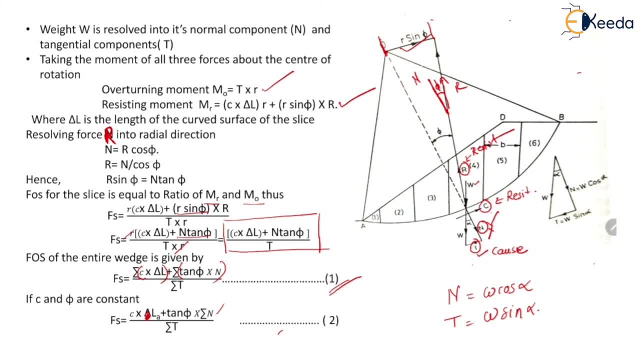 And Summation Of N Is The Total Number Of Slices Divided By Summation Of T. So We Will Name This Equation As Equation. 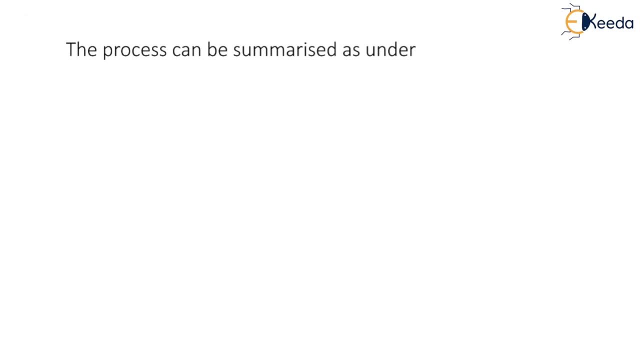 To Determine The Value Of Safety. So, In Short, The Process To Determine The Factor Of Safety Using Swedish Circle Method Can Be Summarized As: 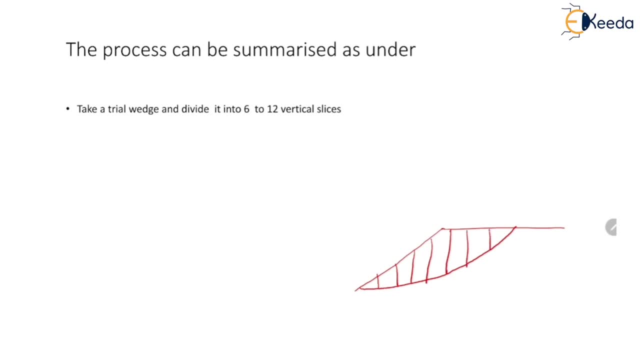 Entered. The First Step Is To Determine The Weight Of Each Slice And Its Line Of Action. So Weight Will Be Equal To Area Into Density.